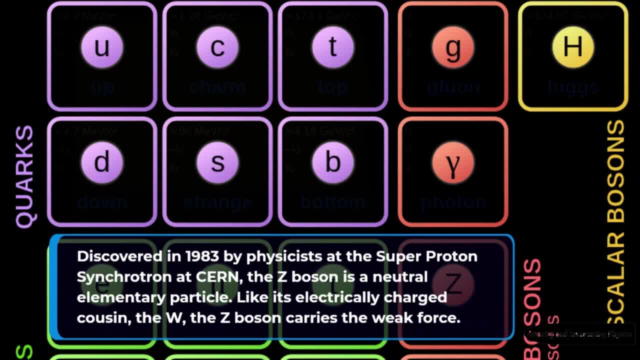 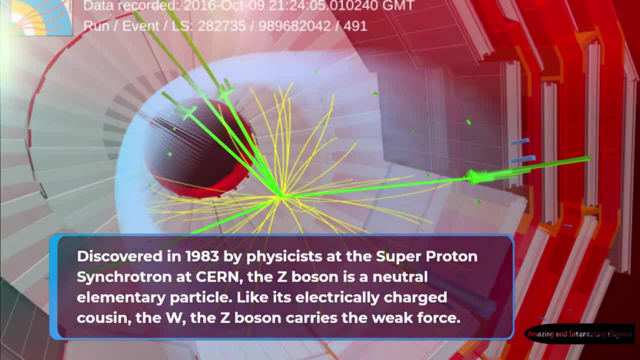 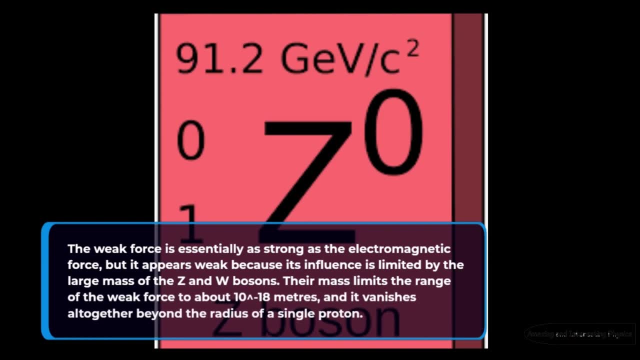 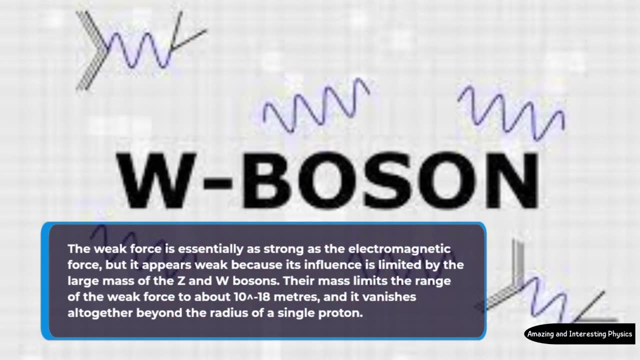 Like its electrically charged cousin, the W, the Z boson carries the weak force. The weak force is essentially as strong as the electromagnetic field, But it appears weak because its influence is limited by the large mass of the Z and W bosons. 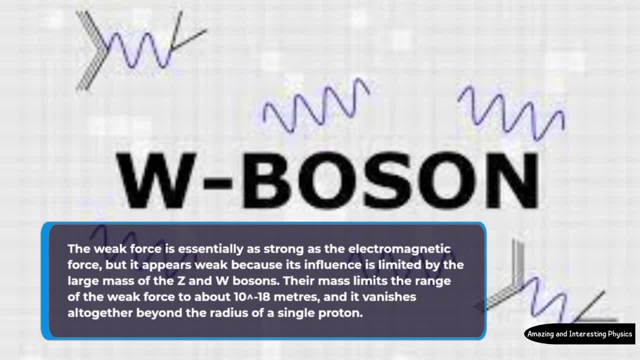 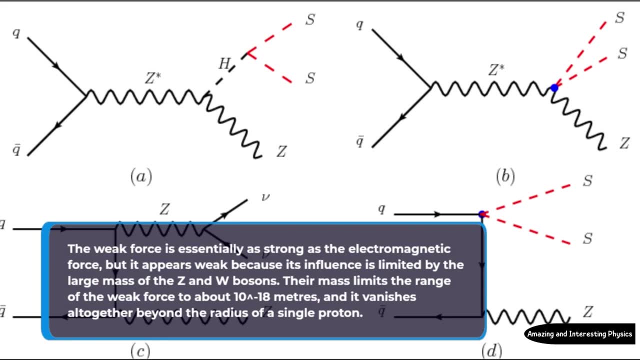 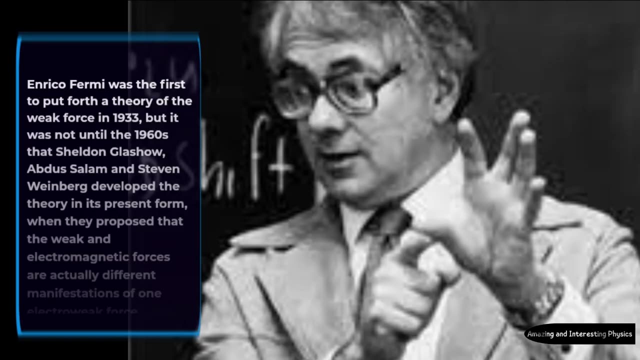 Their mass limits the range of the weak force to about 10 to 18 meters and it vanishes altogether beyond the radius of a single proton. Enrico Femi was the first to put forth a theory of the weak force in 1933. 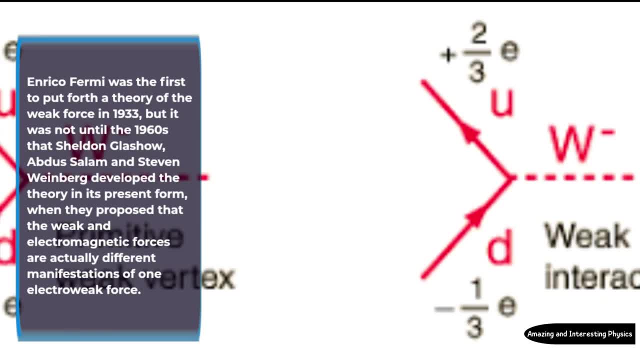 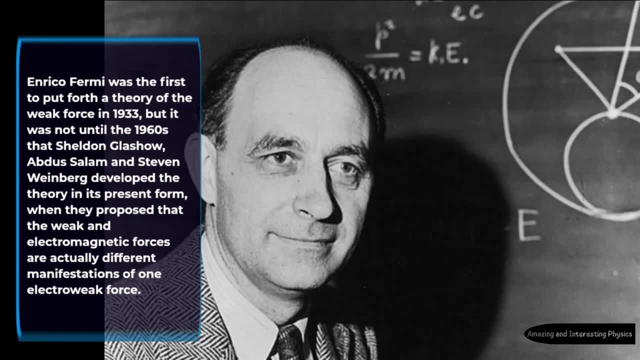 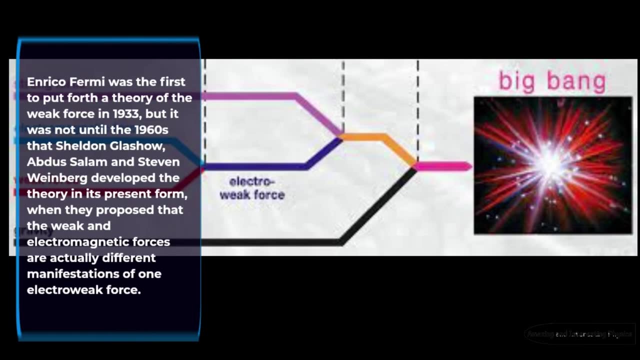 But it was not until the 1960s that Sheldon Glashow, Abdus Salam and Steven Weinberg developed the theory in its present form, when they proposed that the weak and electromagnetic forces are actually different manifestations of one electroweak force. 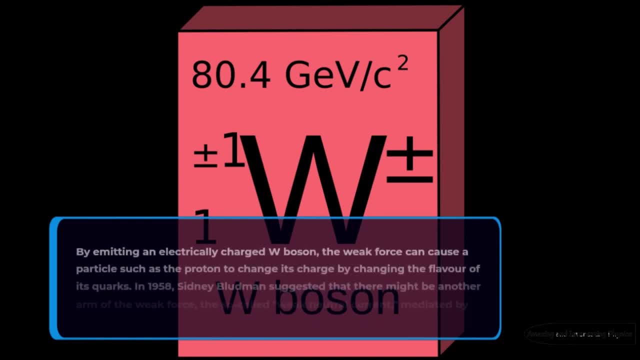 By emitting an electrically charged W boson, the weak force can cause a particle such as the proton to change its direction. The weak force can cause a particle such as the proton to change its direction. The weak force can cause a particle such as the proton to change its direction. 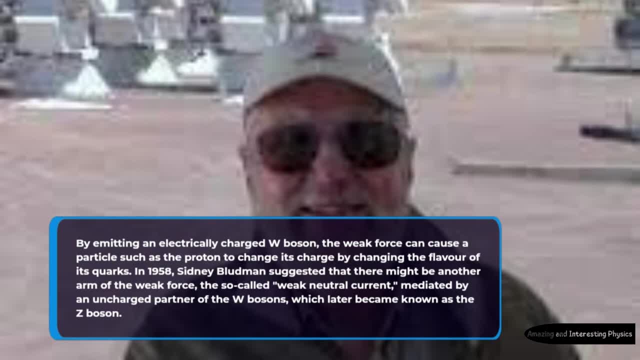 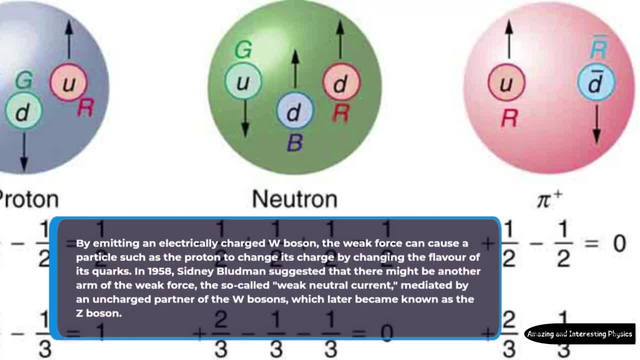 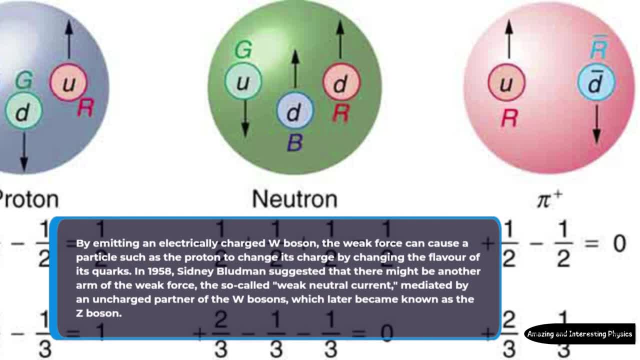 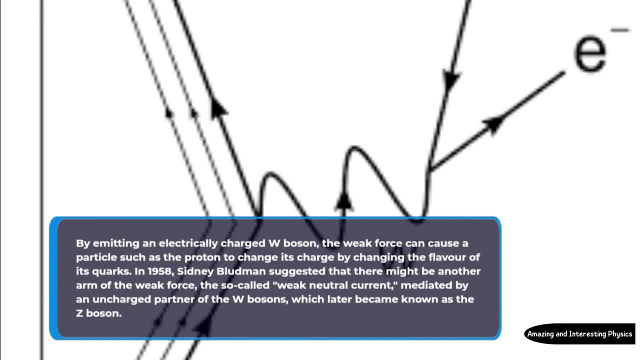 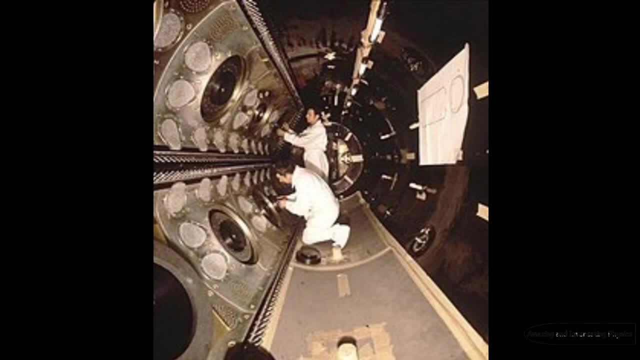 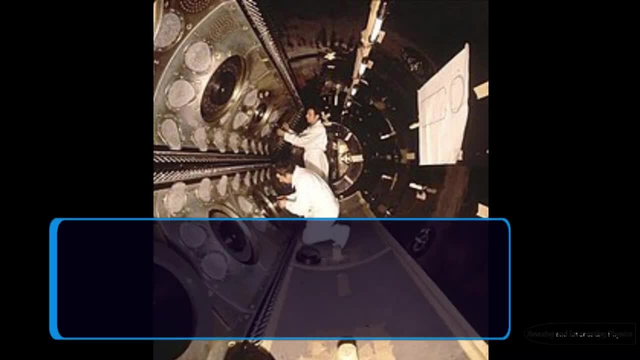 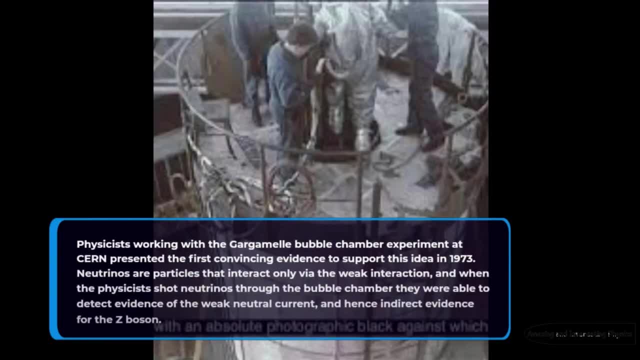 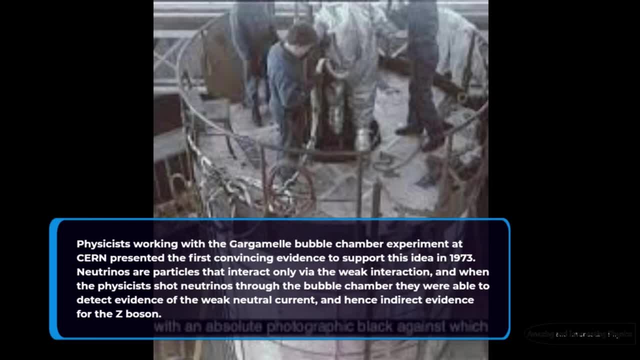 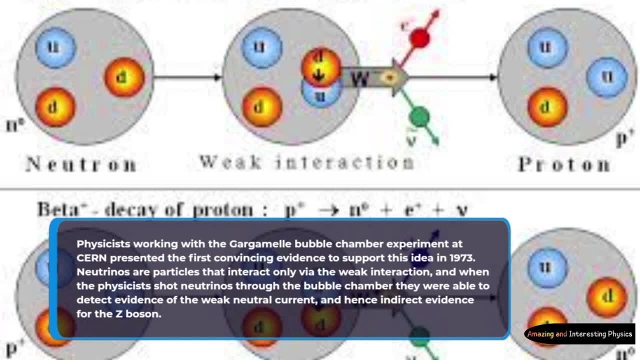 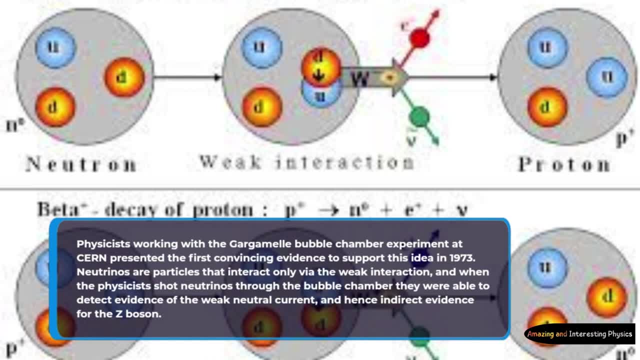 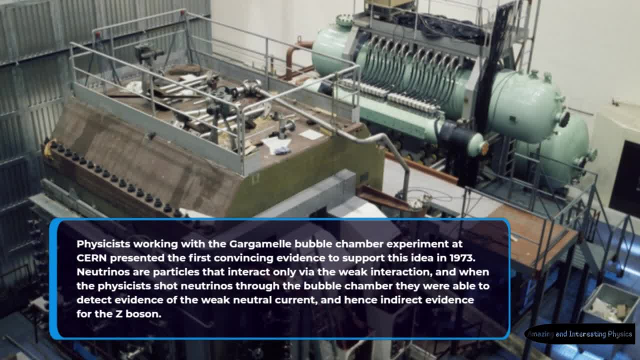 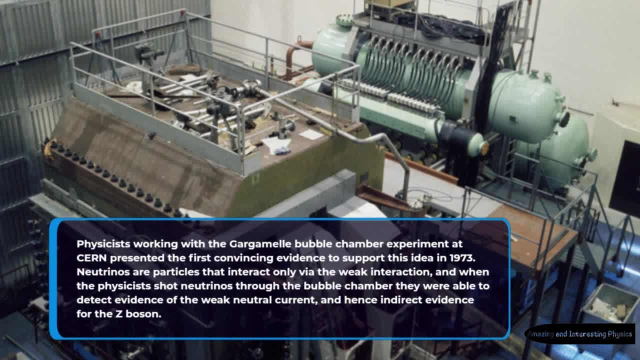 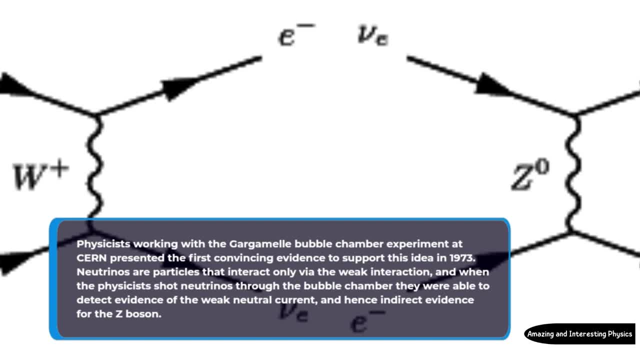 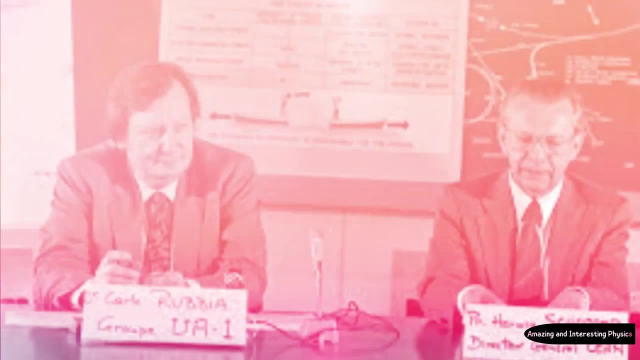 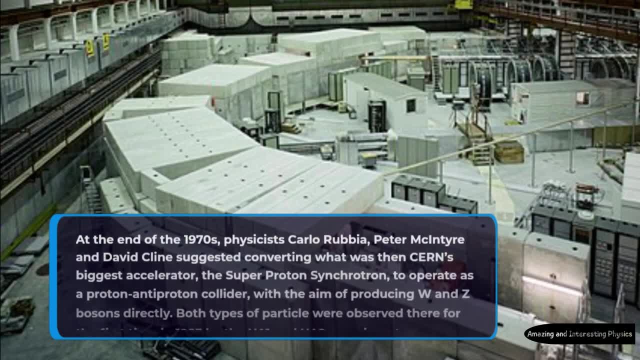 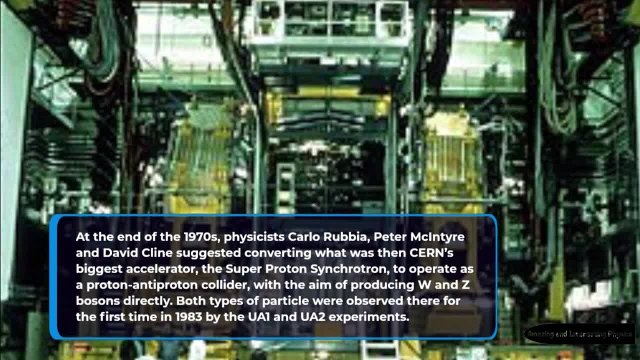 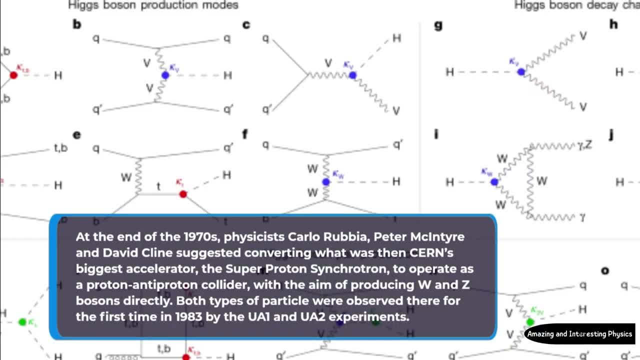 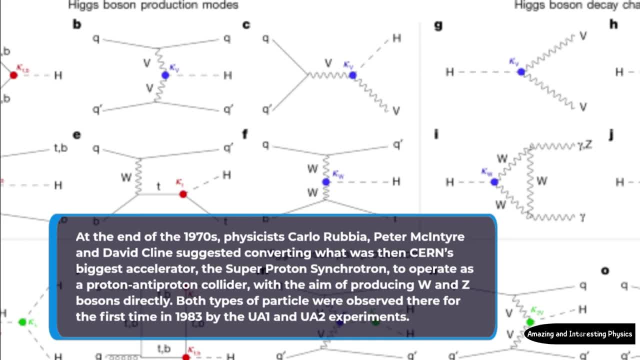 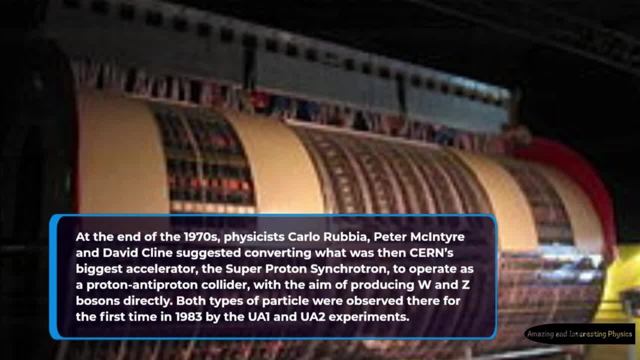 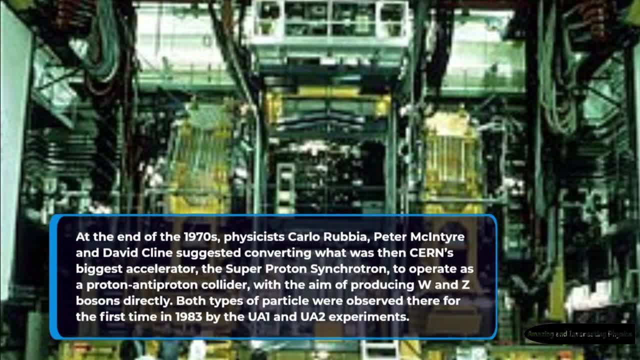 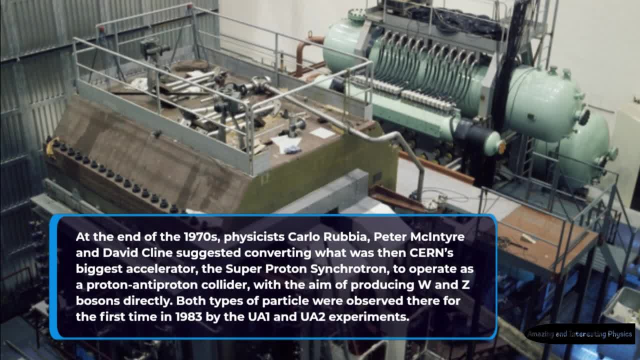 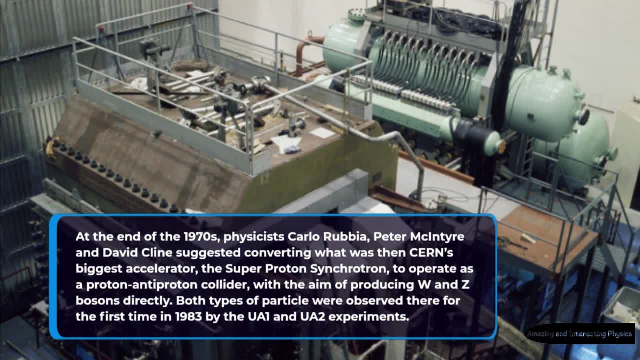